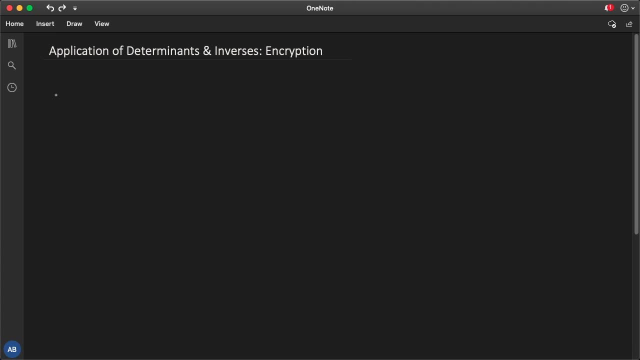 and matrix determinants and so on. So we'll start off by a theorem. I'm not aware of the name of the theorem. If you know the name of the theorem, kindly post it down in the comment section below. So the theorem goes as follows: If a is in z, n by n, what is that? It's the set of integers, and 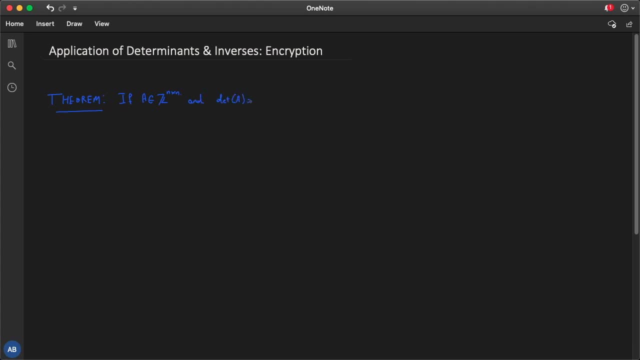 the determinant of a is restricted to plus or minus one, then we can say something about the inverse of a. First of all, it exists. Why? Because the determinant of a is not zero. And second, and most importantly, a inverse is also in z, n by n. That said, a inverse is also a matrix with integer entries. That's super important And it is trivial. for the particular case, n equal one, right. So for n equal one, what do we have? 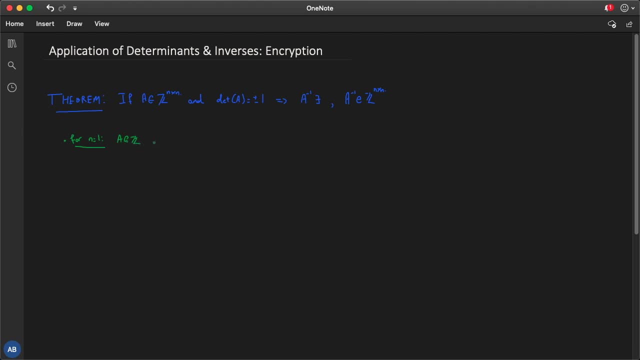 a is a scalar right, An integer, scalar And determinant- of a is plus or minus one. That said, a is either plus or minus one, right? We've got no other case. So the inverse of a exists, of course, it's not zero. And second of all, the inverse of a is also an integer. Why One over a is one over plus or minus one? That said, a is either plus or minus one, Right, We've got no other case. So the inverse of a exists, of course, it's not zero. And second of all, the inverse of a is also an integer. Why One over a is one over plus or minus one? That said, a is either plus or minus one, Right, We've got no other case. So the inverse of a exists, of course, it's not zero. And second of all, the inverse of a is also an integer. Why One over a is one over plus or minus one? That said, a is either plus or minus one. That said, 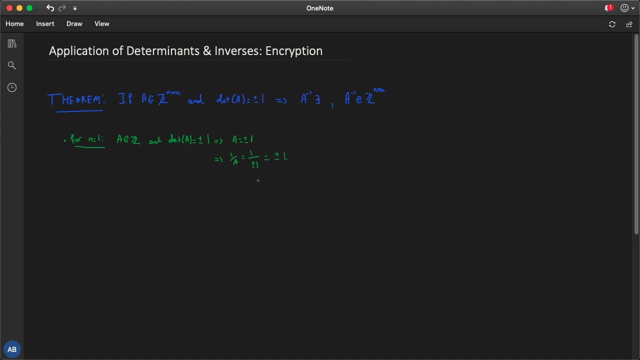 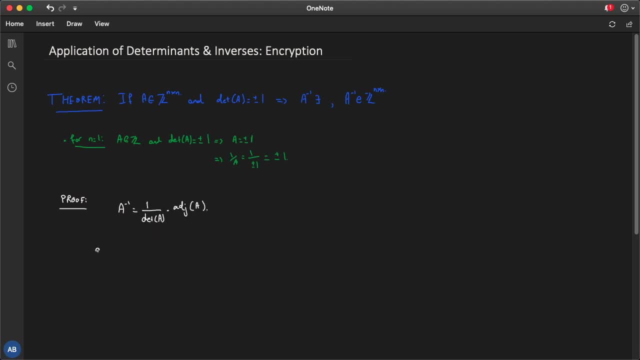 Of a. So, as a quick revision, what is the adjoint of a? It is a matrix containing the cofactors of a. So actually it is the transpose of the matrix containing the cofactors of a. So it takes the following form: where each component cij is computed by a suitable sign minus one to the power i plus j multiplied by the minor ij, That is a determinant right Obtained by emitting the ith and jth. 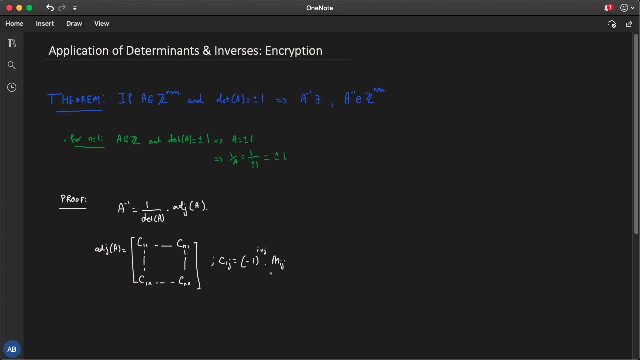 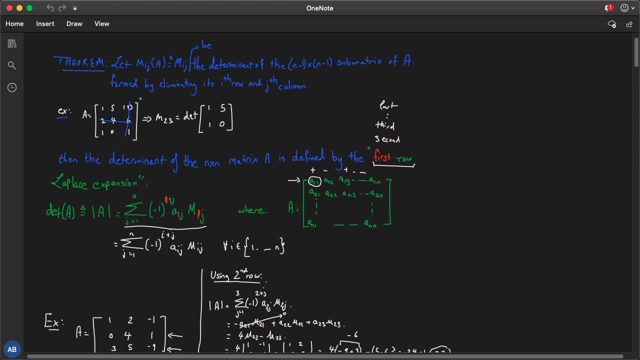 i throw and jth column of a. What can we say about mij? Well, we saw in previous lectures that mij is a determinant of the n minus one by n minus one submatrix of a formed by removing its. i throw and jth column. So if we have a matrix of all integers as such, what can you say about all the minors of a? They're also integers, Why? 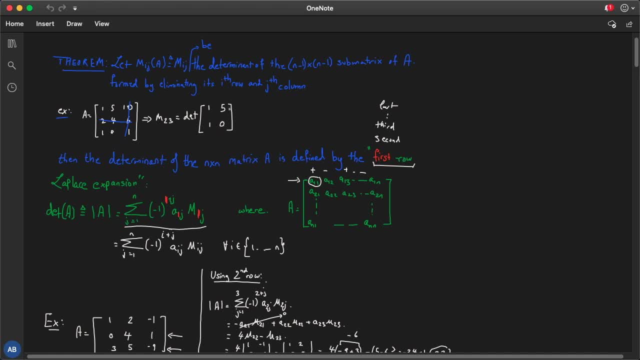 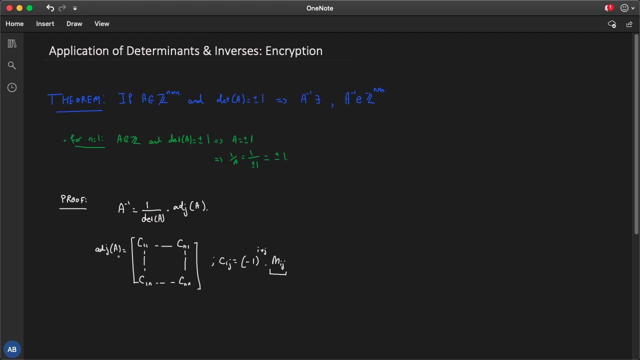 Because they're obtained by simple product and sums of integers, And we all know that if you multiply two integers or add two integers, subtract two integers, the result is also an integer. That said, the minors of a matrix containing integers are also integers. Why do we care? Because that means the adjoint of a will be also a matrix of all integers. Okay, why do we care about that? Well, 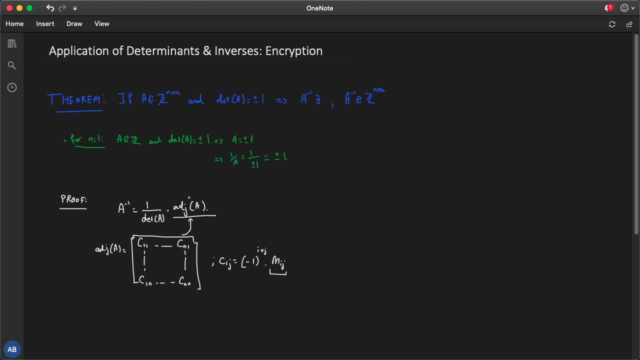 using this piece of information, we know that the inverse of a is a matrix in zn by n, divided by the determinant of a. Well, in this particular case we've got that the determinant of a is either plus or minus one, And hence you're multiplying with either a plus or minus one. So if you're multiplying an integer, any entry of the adjoint of a, with either a plus or minus one, it is also going to be an integer, And hence the inverse of a is also an integer. 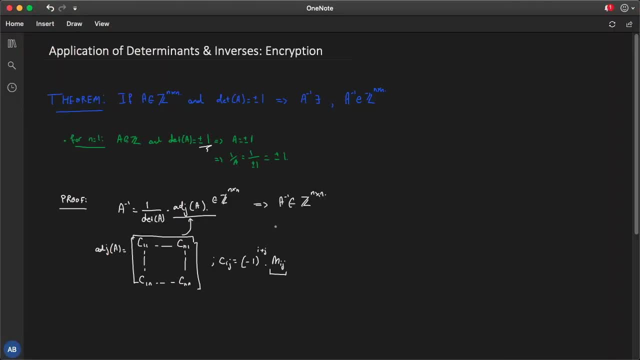 matrix of all integers right And the proof is done. So back to the application over here. that is on encryption. Now, keep in mind that encryption and decryption is a very big topic And a lot of well known researchers put a lot of effort in this field Because of the usefulness of encryption. For example, this is due to the explosion of financial transactions on the internet. So 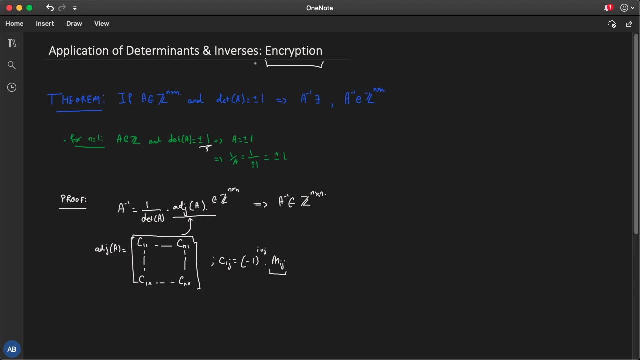 I don't know if you already knew that, But Bitcoin uses a lot of encryption while validating a certain transaction. It's not as simple as it seems. So say, I want to send someone a Bitcoin. Well, it's not as simple as just sending a simple message. right, There's a lot of you know, forward backward exchange of keys and many, many sophisticated stuff going on before sending this Bitcoin. So one way of 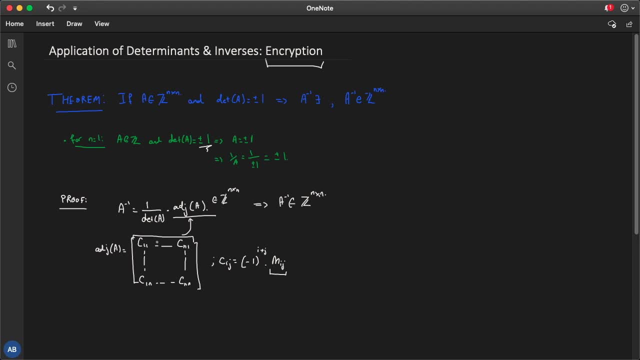 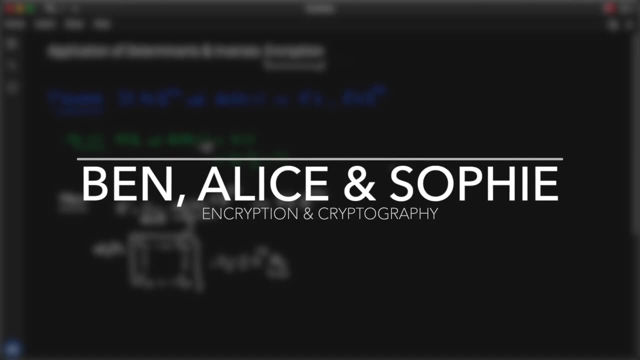 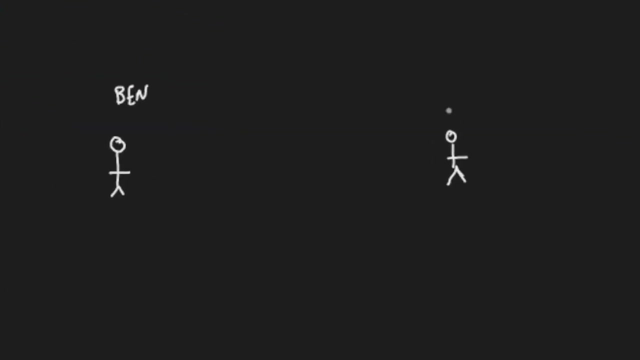 encrypting a certain message is to use inverse matrices. And when I say inverse, I mean let me show you what I mean. So let's say, I've got Ben over here, who is in connection with, let's say, his wife, Alice, right, And they frequently exchange messages in the form of matrices. Let's put it that way, Because that's what it is. you can form any message, you can stack it in a form of a matrix. 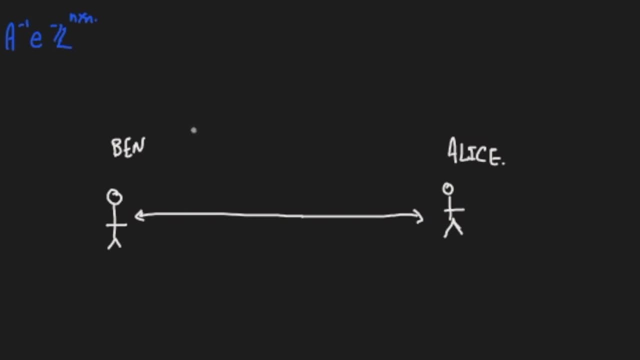 So let's say a message is represented by a matrix, A. So A is a square matrix representing the message. So Ben and Alice are happy, they're sending messages, they're talking to each other- they're in a long distance relationship, I don't know. So they're happy, they're sending messages and each one is understanding the other. Well, one day, an eavesdropper that goes by the name of I don't know, Sophie, 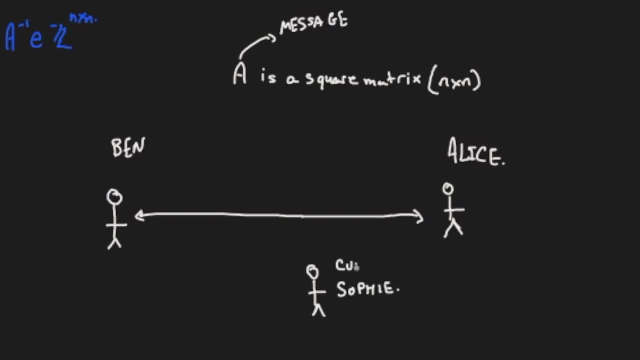 she's Curious Sophie. call her Curious Sophie. What Curious Sophie decides to do is, you know, eavesdrop. She found a link between two people, Ben and Alice, and she decided to eavesdrop. Well, Sophie is a human being and it happens that she can understand the matrices of the form A. So if Ben is sending Alice a matrix A, not only Alice receives A, but also Curious Sophie does So. 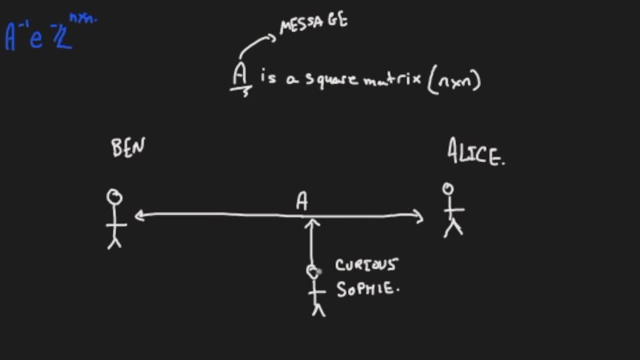 there's a spy over here, there's an intruder, And this intruder is not in the favor of Ben nor Alice. Well, one time Ben found out that there's a curious person grabbing all the matrices A and knowing what there's the conversations between Ben and Alice are, And Ben decided to take action and to watch my courses. And it happened that Ben and Alice were. 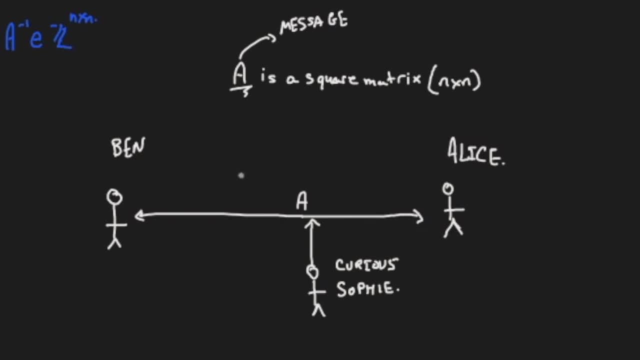 Ben and Alice were watching my previous courses on determinants and inverses and decided to use that knowledge. Well, what did they decide to do? Well, they decided, you know. they said: well, whatever, we'll just sense rectangular matrices. So instead of A, we'll be sending B. So this time a message. 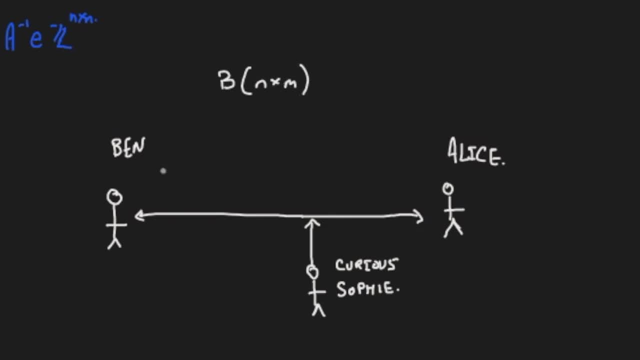 takes a form N by M, and you know Ben and Alice will exchange B. Sophie could also understand what B is. So Ben didn't do anything innovative over here and nothing useful. Well, Alice came up with an idea that you know: instead of you sending any matrix of any size, you're going to send me a. 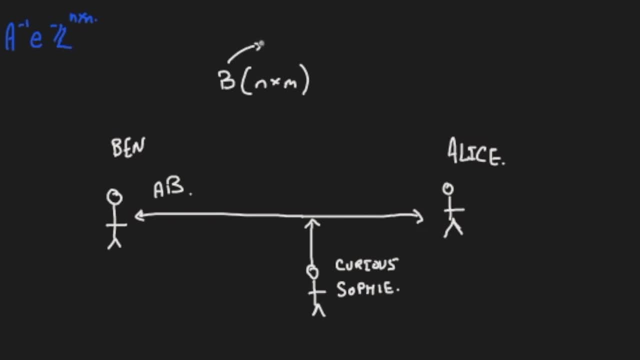 matrix AB where A. So right now, B is the message and A is a certain key. A is a square matrix and it will be representing The so-called key. Why is it a key? Because Ben knows about A and A also happens to have an. 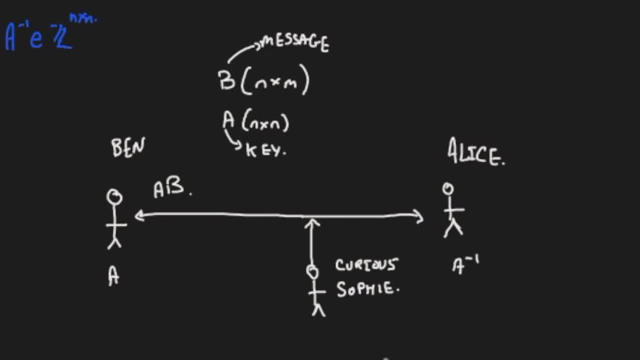 inverse. So Alice knows about its inverse, A inverse. Okay, curious Sophie didn't watch my lectures and she doesn't know anything about matrix, inverses or determinants or whatsoever. So Sophie will just bluntly take AB and understand it as she wants. So AB is also of size N by M. So while Ben sends an AB, a matrix AB, curious Sophie receives an AB. 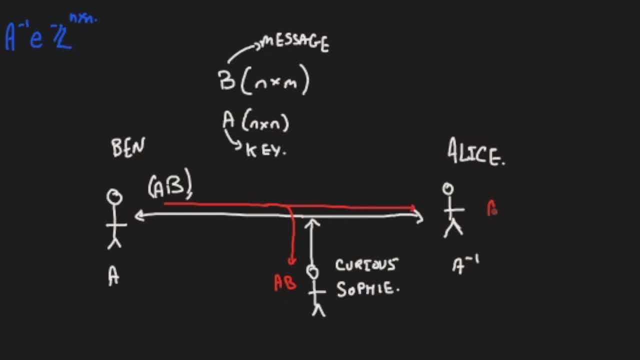 and so does Alice. But what Alice does is take this AB pre-multiplied by an A inverse use, the associative property of matrix products. that is, she knows that A inverse A is the identity I, and hence we'll end up with the desired message B. 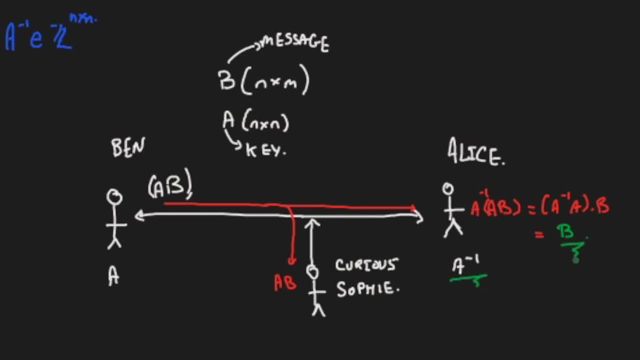 So knowing A inverse will give you the correct message. Not knowing it, in the case of curious Sophie, will give you the wrong message. AB. So in that case, we have encrypted the message using the matrix A, so that the receiving end, that is, Alice, will need to know A inverse in order to decrypt. 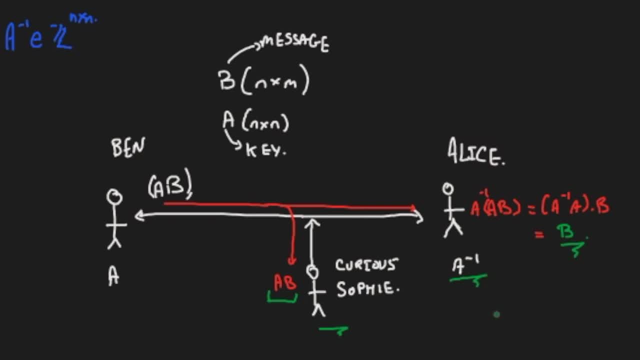 the message B. Now, keep in mind that whenever an undesired intruder, as is the case of Alice, is curious, Sophie finds A, let's say, curious. Sophie watched my lectures and she knows about this fishy inverse matrix right. Well, what people usually do is they change A frequently, more frequently. so 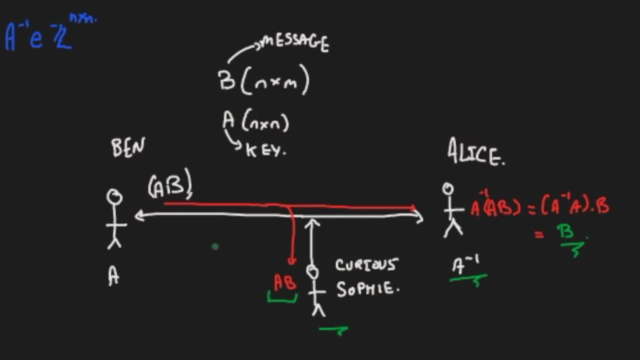 that the sender and receiver both know about this A and make it really hard for any other receiving end. So we should have a mechanical way of, you know, generating simple matrices A which are both invertible and have simple inverses, Because we know that in practice. 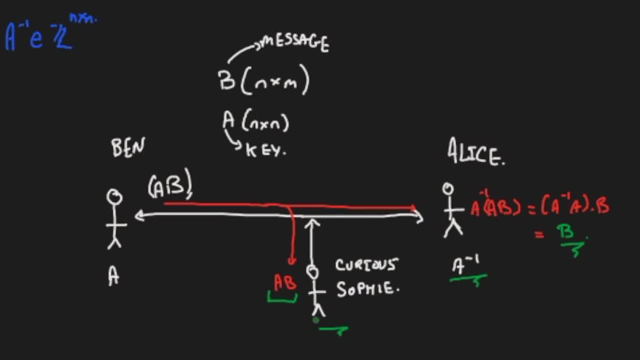 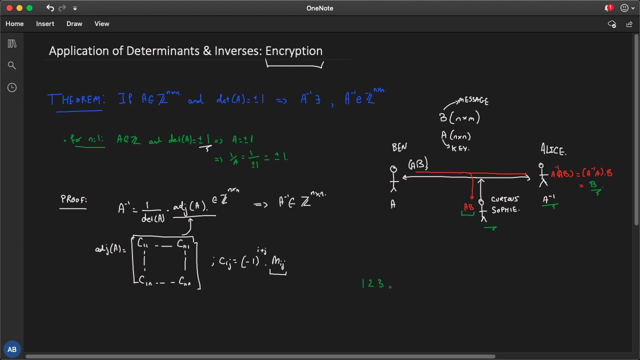 the inverse of a matrix involves fractions which are not easy to to send electronically. Fractions take a large amount of data. So in case you don't know what I mean, so let's say you want to store an integer, one, two, three up to- I don't know- 64. Okay, so how? 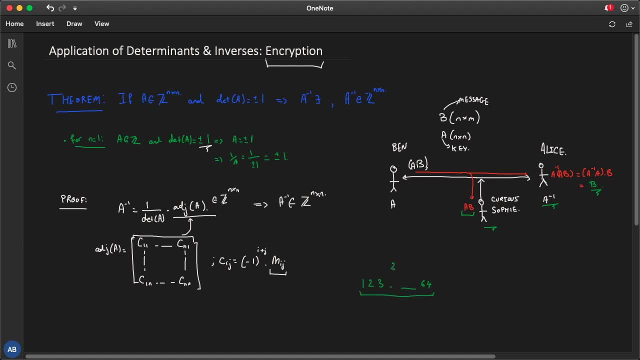 many bits do you need to represent those numbers? You need eight bits. so two power eight to represent numbers going from one to 64.. So you need eight bits, that's it. that's all the memory you need, Whereas if you want to represent fractions, it might go a lot more than that. Why? Because 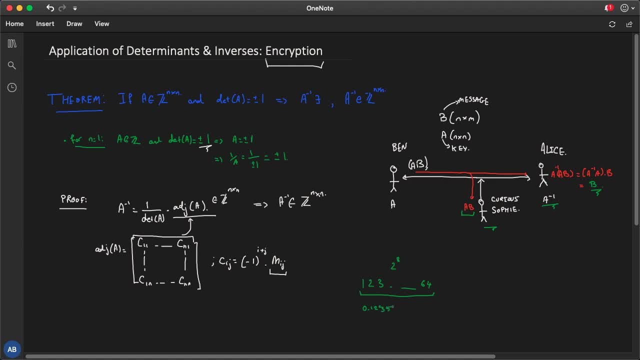 representing 0.1235, for example, is not the same as representing what you see in front of you here. This might need way more bits than just eight. So you can see that the matrix inverse is not that straightforward. It's not favorable in practice. 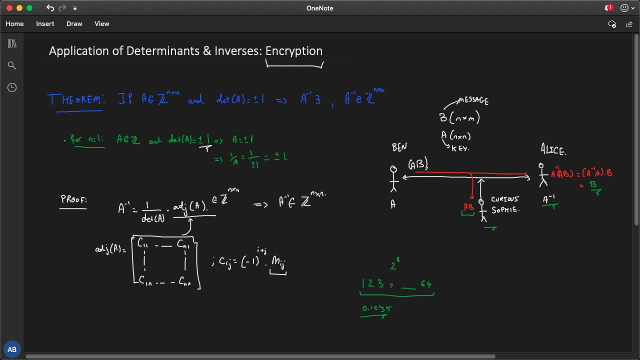 So the optimal solution here would be to have both A and its inverse in integer form, And that's where this theorem comes in place. So this theorem will be useful to generate such classes of matrices. So one practical way is to start with an upper triangular matrix with entries that are either 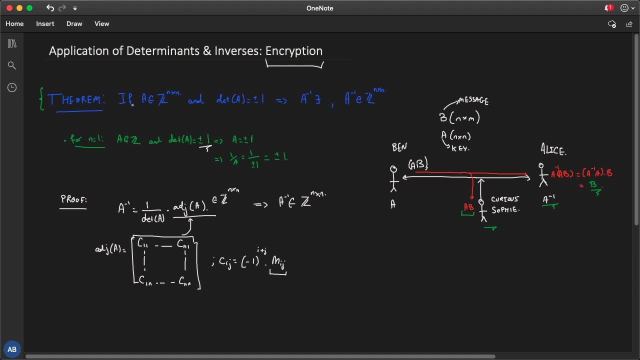 plus one or minus one on the diagonal and integer entries. Why do we say that? Because if let's say this is my A, Let's say n is three, for simplicity. So we, you know, plus one over here, minus one over here, plus one over here, zero, zero, zero and really. 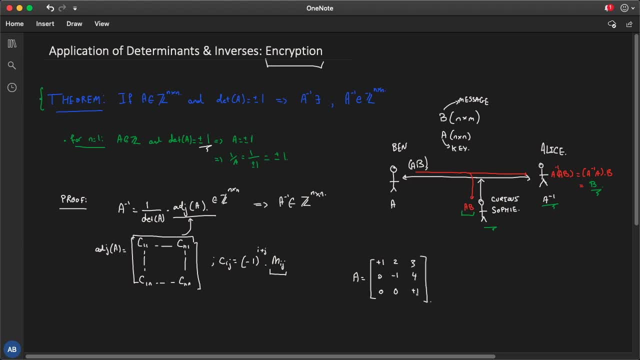 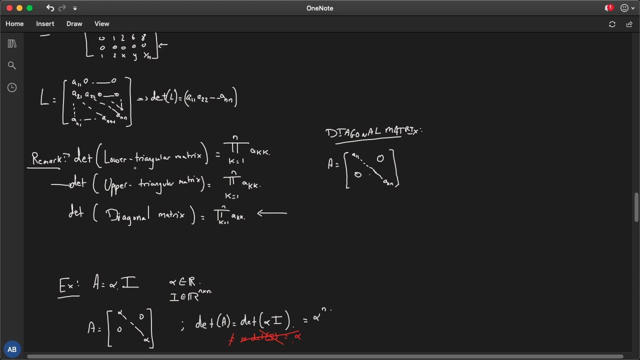 any integer over here. two, three, four. let's say Why did we impose this structure? Because we know that the of triangular matrices, whether it's upper or lower, is just the product of its diagonal entries. Well, keeping this piece of information in mind, 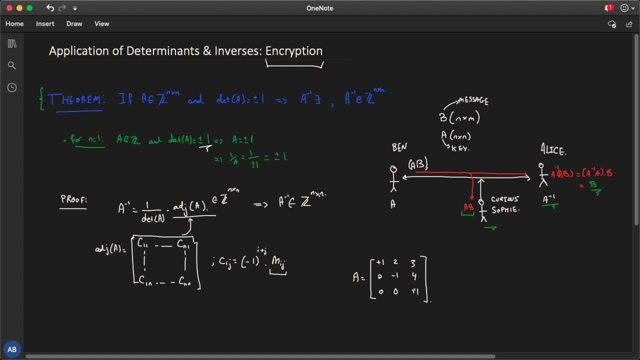 multiplying either plus or minus ones here on the diagonal will give you a determinant that is either plus or minus one, And throwing in integers over here will preserve A to be found in the set ZN by N right. That said, the inverse of A will also be in ZN by N. 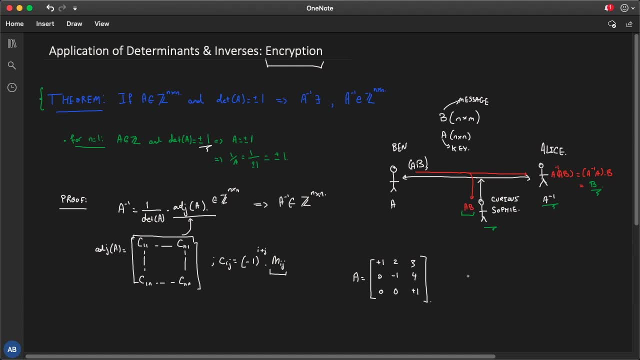 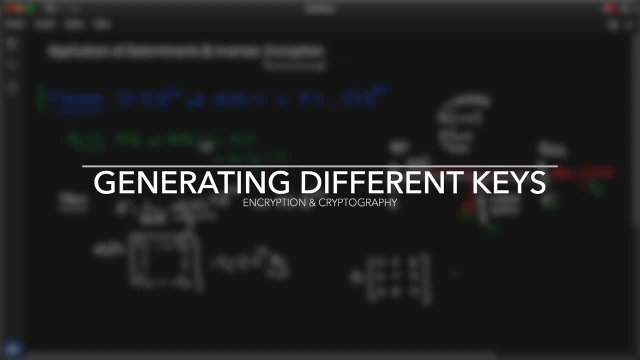 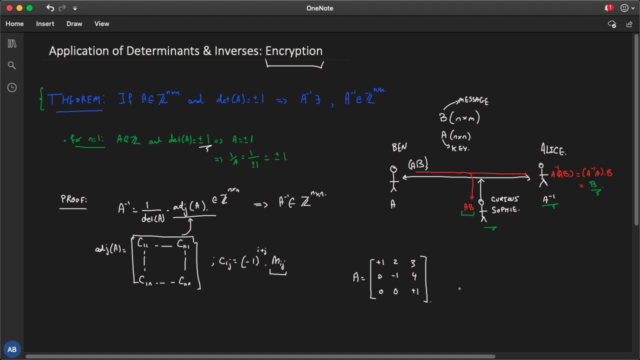 and hence we avoid the computation of, you know, fractions Now. furthermore, we use elementary row operations to alter the matrix. We do not multiply rows with non-integers, that is, we'll only be restricted to integers and adding a multiple of one row to another. 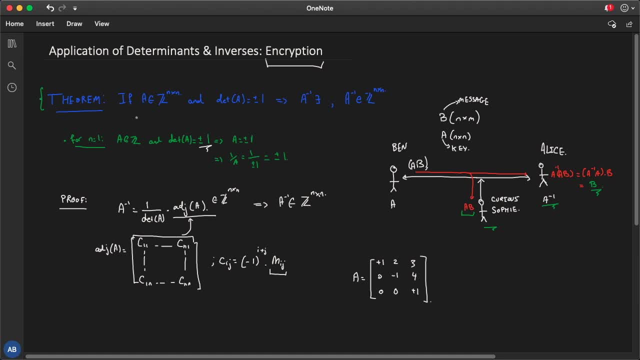 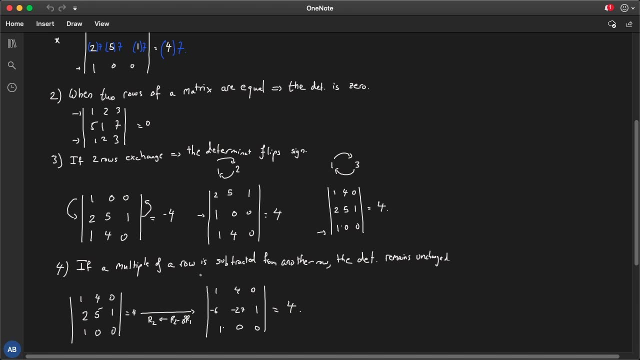 does not change the value of the determinant. We saw that in the previous lecture right And in particular here. if a multiple of a row is subtracted from another row or added doesn't make any difference. the determinant remains unchanged. Extra information over here are: if you flip two rows, 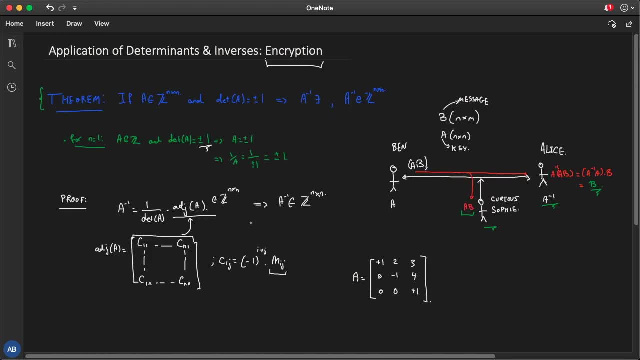 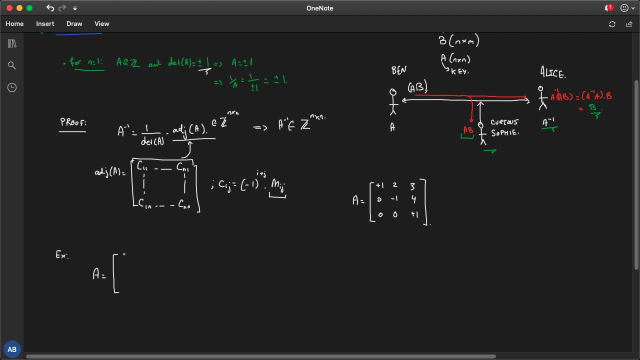 the determinant flips sign, and yeah. So let's give an example on what I mean. Consider that we've got a matrix A, that we load the diagonal with either plus or minus one as such, impose it to be upper triangular and just throw in some random- you know- integers over here. 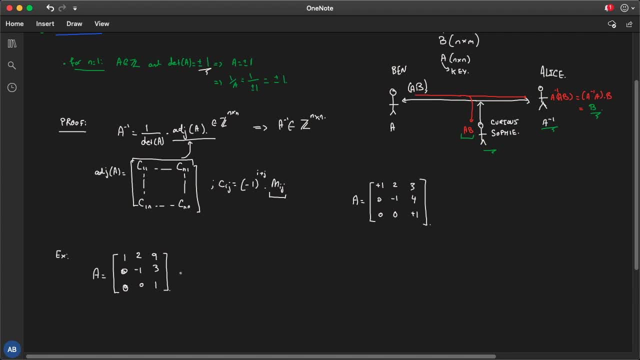 Let's say two, nine and three. Well, let's do some row operations over here. Let's say: in R2, I put in R2 plus R1.. That said, the first and third rows remain unchanged, whereas the second row remains unchanged. 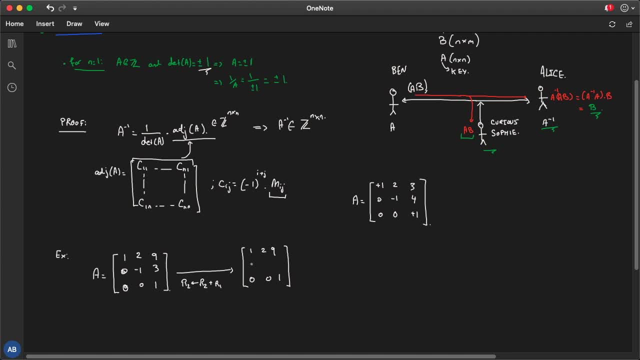 So the second row becomes: we start: one plus zero is one, two plus minus one is also one, and nine plus three is 12.. Do the same thing for the third row, that is, instead of R3, plug in R3 plus R1.. 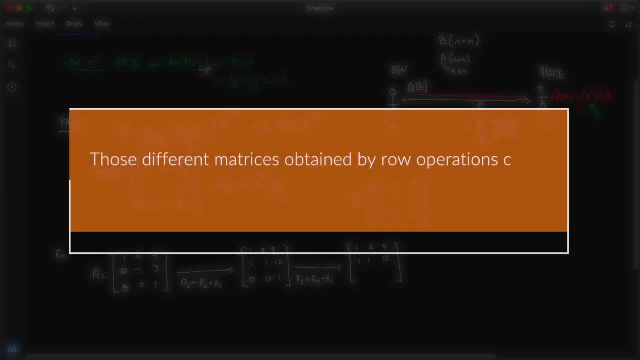 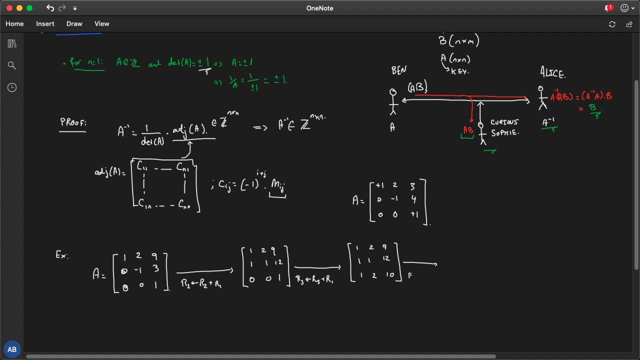 That said, the first two rows remain unchanged, whereas the last row becomes one two and 10.. Now do one more operation on the third row, that is, instead of R3, put in R2 plus R1.. R3 plus R2, the first two rows are unchanged. 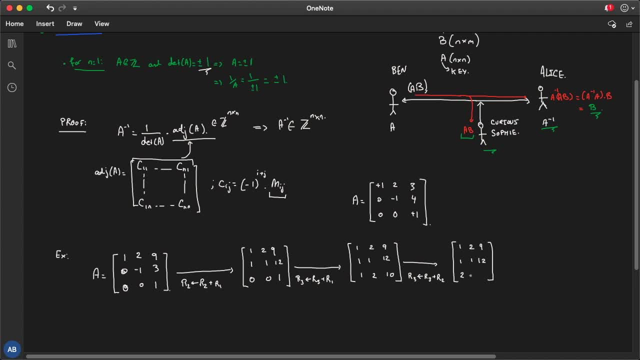 whereas the last row becomes two, three and 22,. okay, So, if you're noticing, we're just doing some random operations, I'll do one more here. So instead of R1, I'll put in R2 plus R3, right? 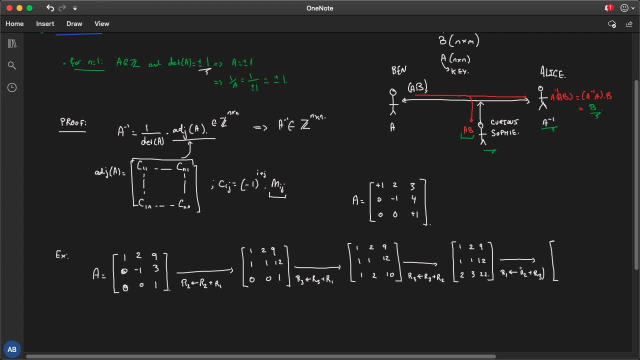 So I'll get, and not just that, I'll multiply this by a minus two and add it to R1.. What we get is the following: So the second and third rows are unchanged, whereas you can go ahead and verify that the first row becomes minus five. 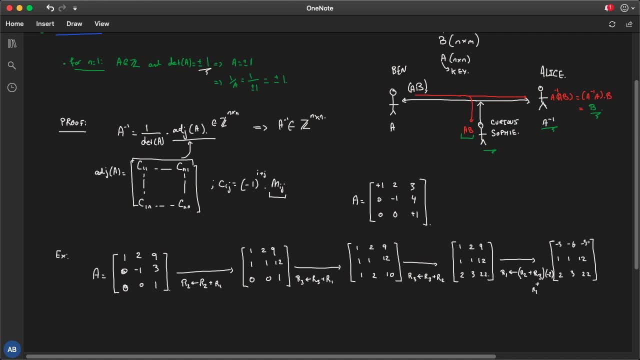 minus six and minus 59, right Now, since we did a bunch of, you know, scaling and adding, we didn't flip two rows. The determinant of A is the same as the determinant of this last matrix over here, So I'm going to eliminate A from here. 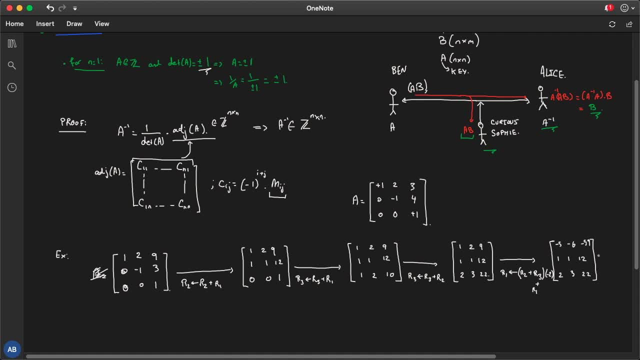 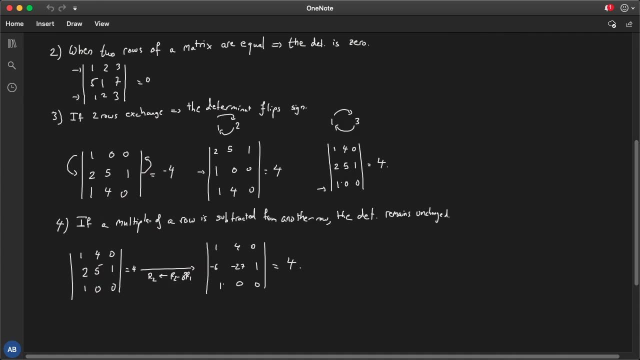 This notation A. I don't want it here. here I want the last matrix to be a. Well, the determinant of a is also minus one as a, because according to property four over here, if a multiple of a row is subtracted or added from another row. 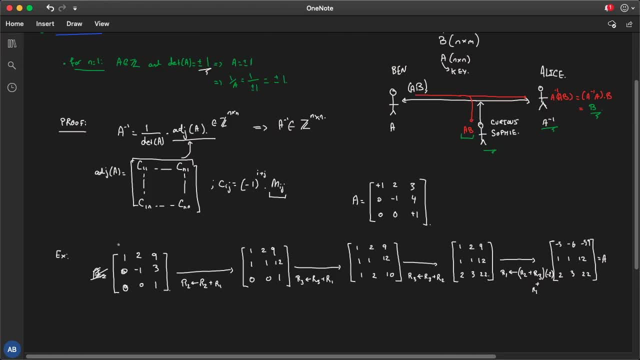 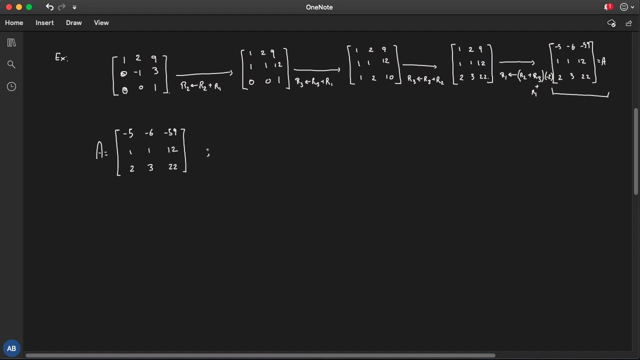 the determinant is unchanged. So the determinant of this first matrix that is minus one is the same as this last matrix, a that is also minus one. So a matrix a. we're going to use this matrix as a key. Okay, so we'll take a to be the last matrix. We know that the determinant of this matrix is: 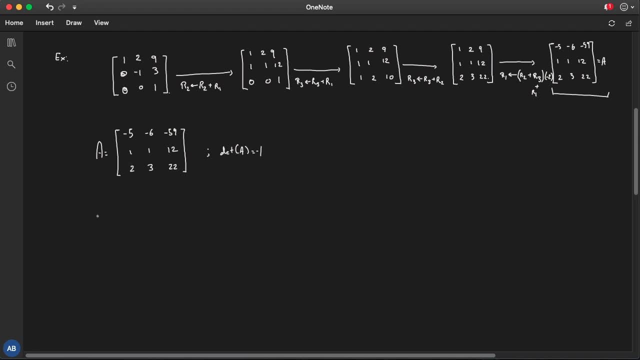 minus one, and hence computing the inverse is easy, Why? All I have to do is compute the one over. determinant is a minus one, so it's a minus the adjoint of a. You do the math, you arrive at the following: So, as you can see, it's a matrix of all integers. and now let's say we've got a message b. 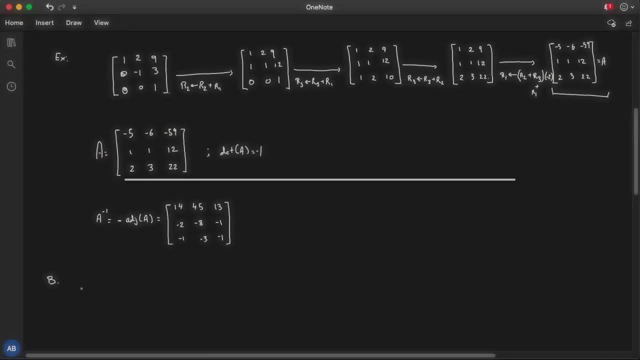 that will reflect the English matrix Today is a good day. So the message today is a good day will be reflected by matrix b. We're now going to put in the characters of today is a good day. this message: m call it m. We're now going to put the characters of m inside a matrix b. No, we're going to associate each. 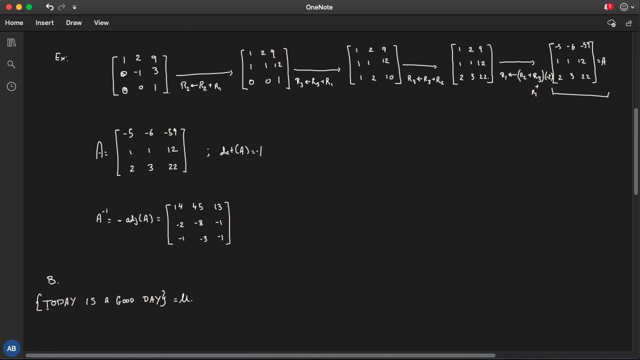 character to a number. We're going to map every character to a number. So an easy way to do that is to associate white spaces, so those by numbers 0, the number 1 to a, the number 2 to b, and so on. So in that way, if we say that, say there's a table with white space, so let's say this is a character and this is the number associated to the character. So white space is 0, a is 1, b is 2, and so on. You get the point. 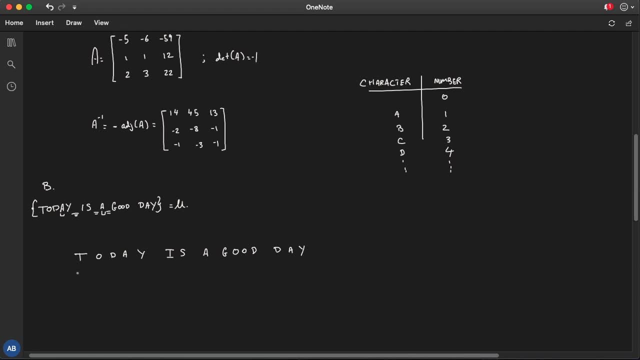 So that case, this message today is a good day, will be map as follows. so t could be minus 10, o could be 8, and so on. Actually, the numbers associated to the characters could be random, so d could be something else, let's say minus 2.. They don't have to be in. 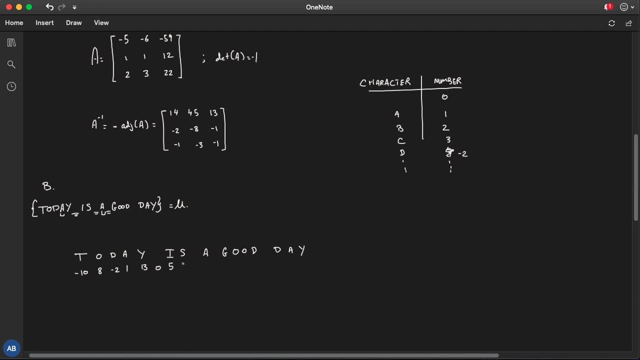 increasing order. okay, i could be 5,. s could be 10,. got a white space here, so 0,. a could be 1, 0, g could be 4, o could be 8, so 8 twice over. here d is again minus 2, we use it here. 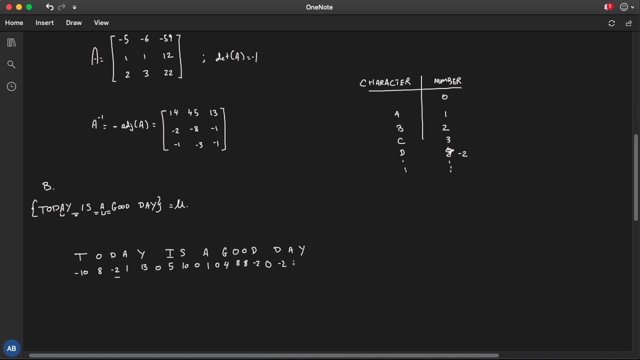 got a white space here: 0,, d is again minus 2, and a 1 and 13.. So if we stack those in a matrix B, how many characters do we have right here? So if we do the math, 1,, if we count them: 1,, 2,, 3,. 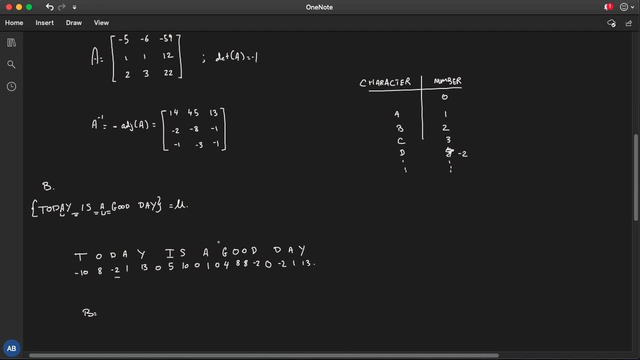 4,, 5,, 6,, 7,, 8,, 9,, 10,, 11,, 12,, 13,, 14,, 15,, 16,, 17,, 18, and 19.. So 19,. we're going to add two more white spaces over here, so 0 and 0.. Why is that So that? 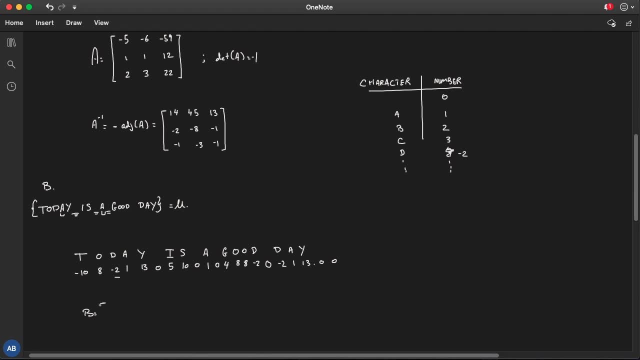 we make the size 21,, that is, 3, could be represented by a 3 by 7 matrix. How Well, all we have to do is grab consecutive 3 numbers and stack them in a column of B. So B would be minus 10, 8, minus 2.. 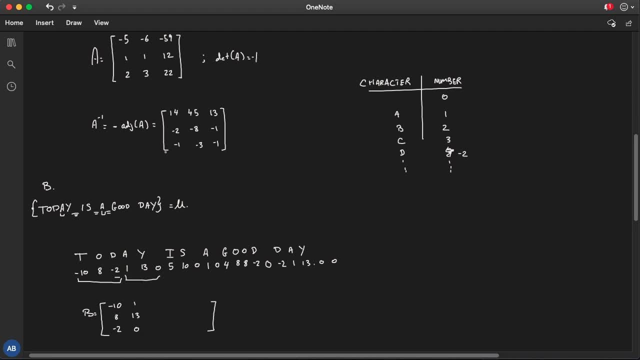 1, 13, 0.. So we need the size of 3 right here, so that it matches the dimension of a, which is 3 by 3.. So we do need the dimension 3 over here. We continue with the stacking 5, 10, 0,, then 1, 0,. 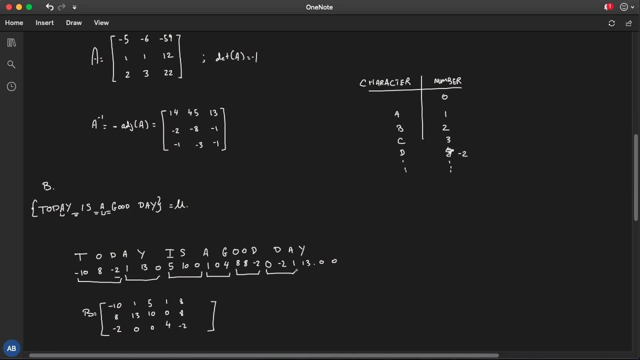 4, 8,, 8, minus 2,, 0, minus 2, 1, and 13, double 0.. Okay, So this is the message that, let's say, Ben wants to send to Alice. So he stacks this: today is a good day. 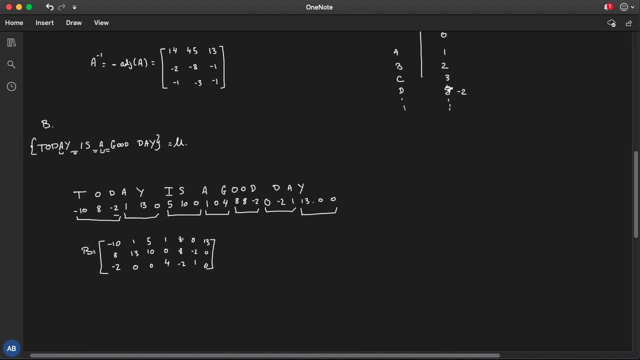 and maybe he's going to send it to Alice, So he stacks this: today is a good day, and maybe he's going to send it to Alice, So he stacks this: today is a good day. he gets this representation of B right, Then, instead of sending B as such. 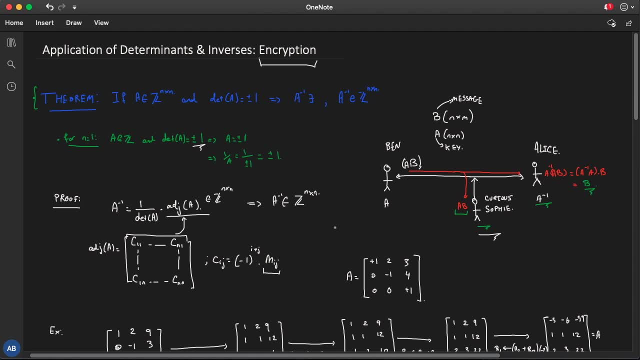 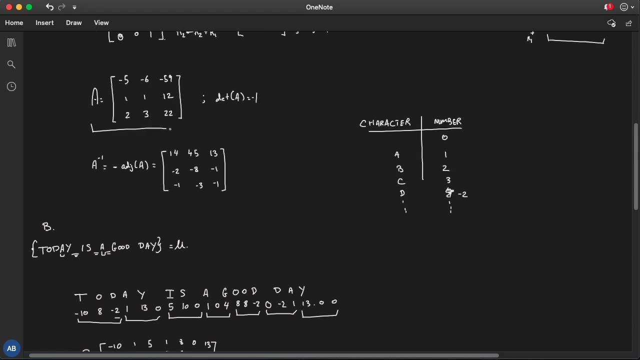 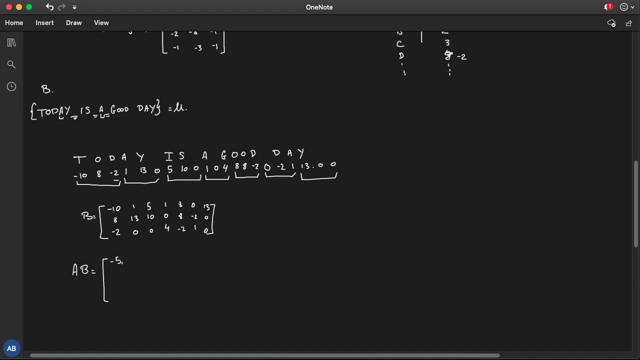 so that curious Sophie does not understand the message. he will instead send A times B. that is the A we just formed over here using a series of row operations. We'll copy it over here. So it's a minus 5, minus 6, and a minus 59, with 1,, 1,, 12,. 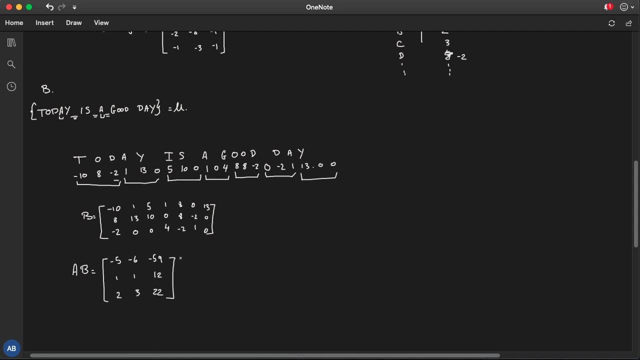 and 2, 3, 22, multiply it with b, that is, you get another 3 by 7 matrix. so you grab every row from here, multiply it with every appropriate column from here to get the entries of ab. that will turn out to be 120 minus 83 minus 85 minus 241, 30 minus 47 and so on. so the encrypted message will: 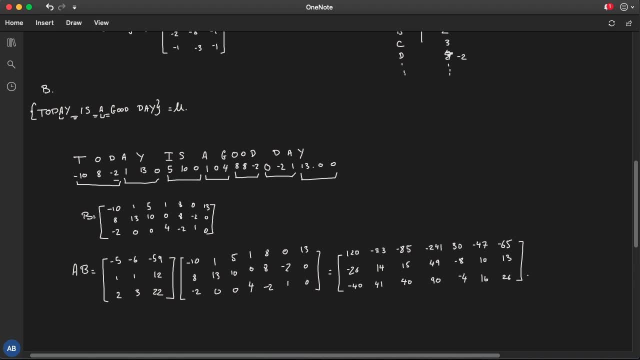 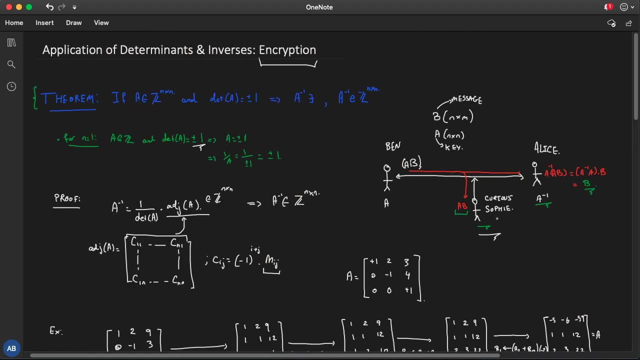 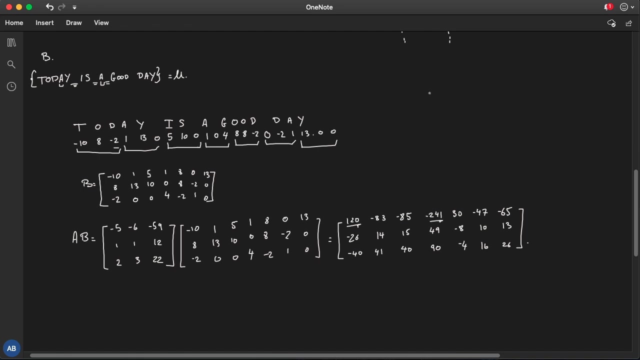 be 120 minus 26 minus 40, then minus 83, 14, 41 and so on. so if, let's say, in the worst case, sophie has the this mapping, the character number mapping, she will not be able to decode the message and, even more than that, she might have really large numbers, such as 120 minus 241, such that you know numbers. 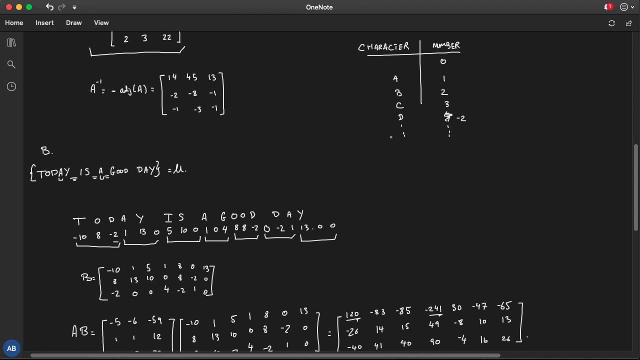 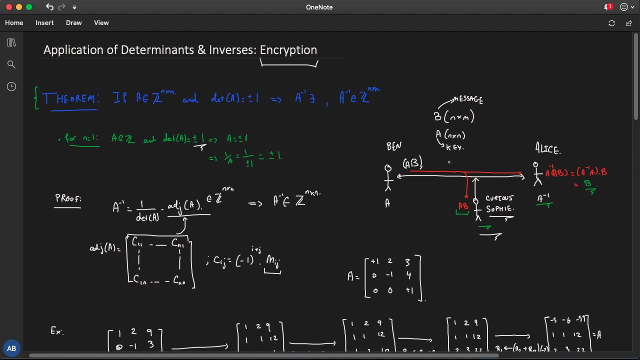 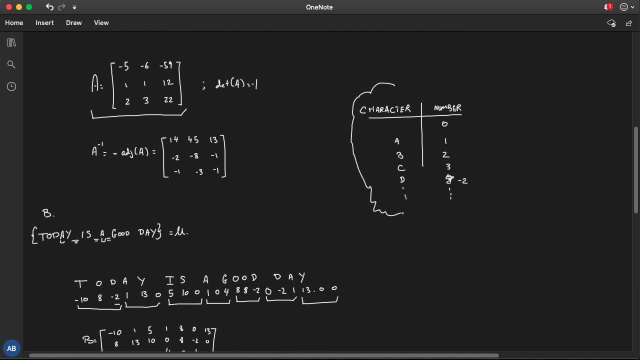 do not have a matching character, right you? so, in that case, sophie will know that there is something fishy going on around here, so you'll know that. oh, ben and alice are no longer using the mapping table between characters and numbers that we have over here, so she'll be wondering: is there any matrix a that is being pre-multiplied? 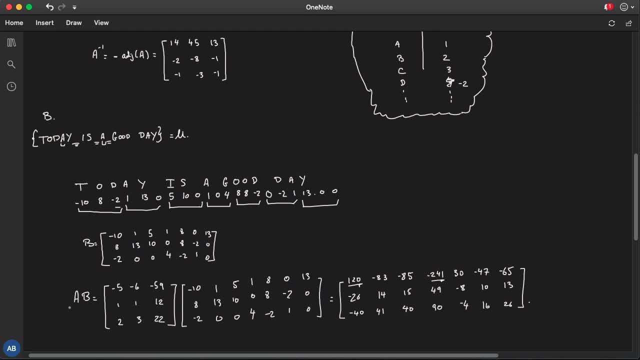 so she will have to try a lot of combinations of a to find out a suitable a that multiplies an appropriate message b to give her this matrix, and this will take her a lot of time. let's say she implements a brute force algorithm to figure out products of the form a, b to give 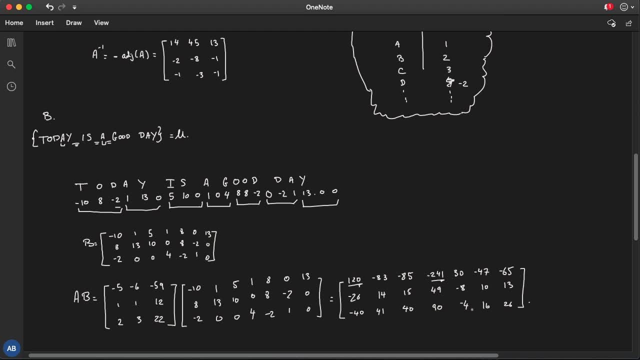 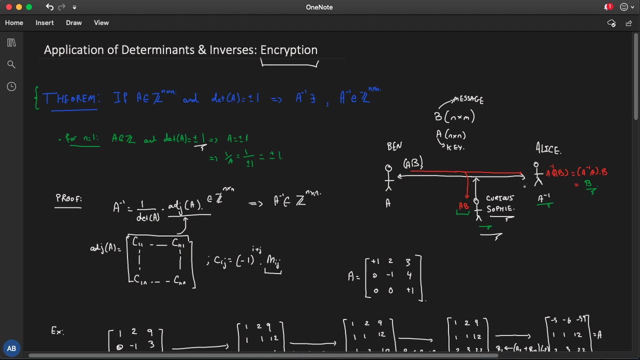 this message over here. it will take her a lot of time, and that time ben and alice would have exchanged all the messages they need. so there you go. so that's the worst case scenario. okay, so that's it for this lecture. we gave an application of determinants. 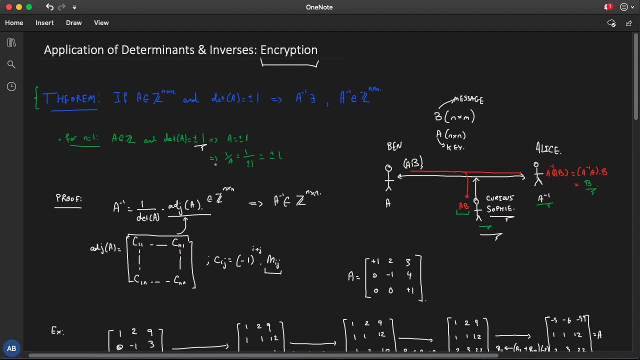 and inverses on the so-called encryption topic Through this theorem over here, that is, if we have a matrix A, that is a matrix with integer entries, such that its determinant is plus or minus one, then the inverse of A is also a matrix with integer entries. Now why is this useful? Well, 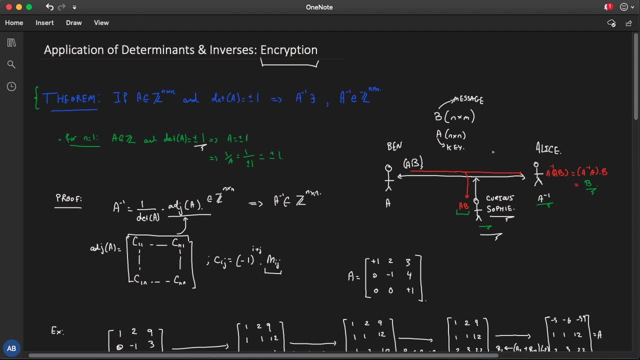 first off, imagine that Ben is sending a message to Alice and instead of sending a matrix B, he sends a matrix AB. Well, Alice will have to compute online an inverse matrix A so as to decode the message AB to matrix B, right? Well, if A was not of this structure, then computing the inverse of A.